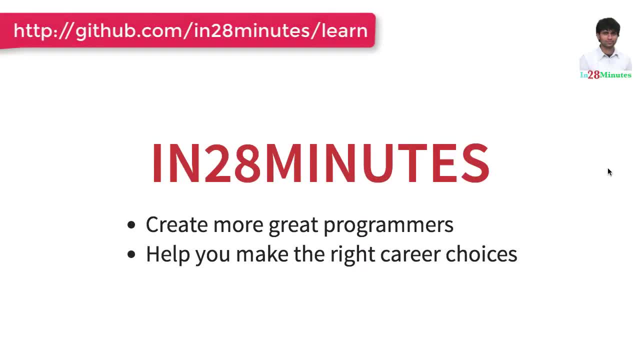 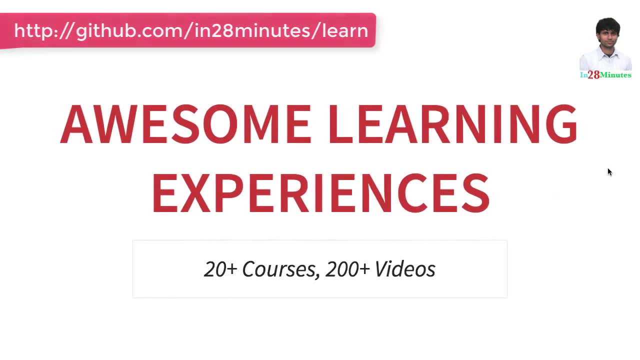 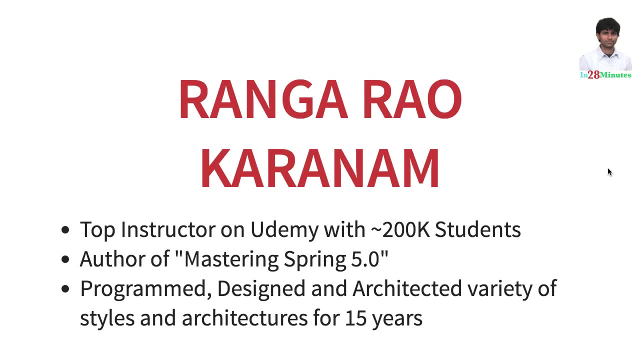 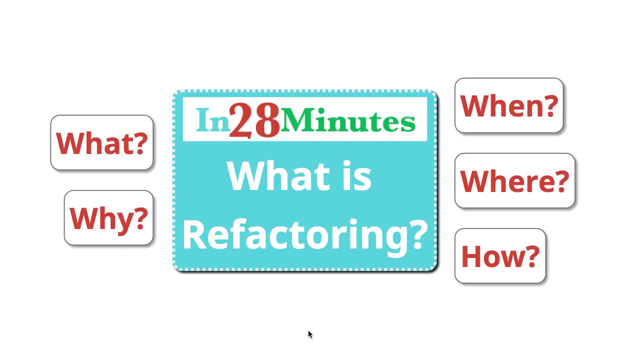 Welcome to this video from In 28 Minutes. Thanks for helping us provide awesome learning experiences to more than 300,000 learners across multiple platforms: Udemy, Safari and PACT. Let's welcome our lead instructor, Rangarao Karnam. In this video, we will be talking about what is refactoring. Why do you need refactoring? 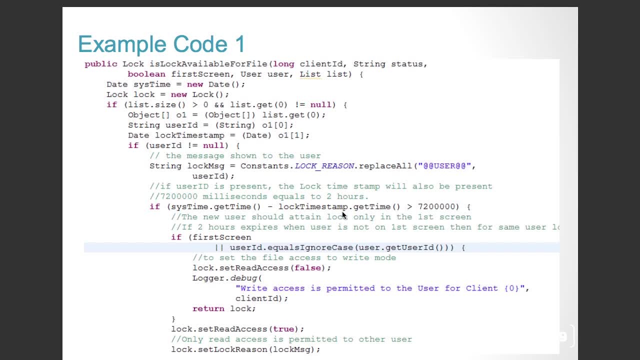 Let's say you end up in a project where you see code like this: Would you love to maintain this kind of code? Is it easily maintainable? Now, let's say I would want to make a change in this specific piece of code. Would it be easy to make change in this kind of code? 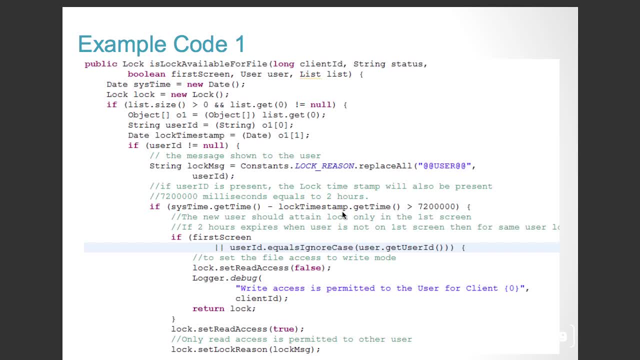 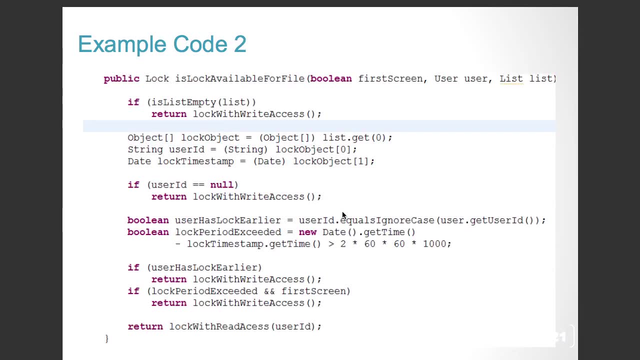 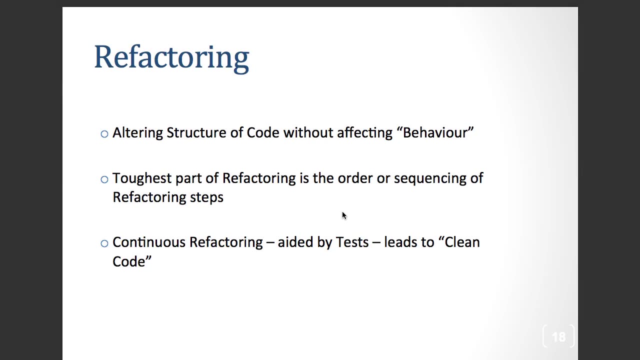 Nope, One of the things I can do is to improve the code without changing the functionality. So I can refactor this. I can change the code but leave the functionality as it is. That is what is called refactoring. Refactoring is all about changing the structure of code without changing the behavior. It. 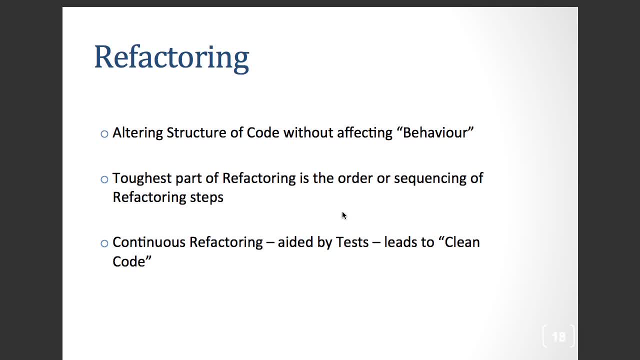 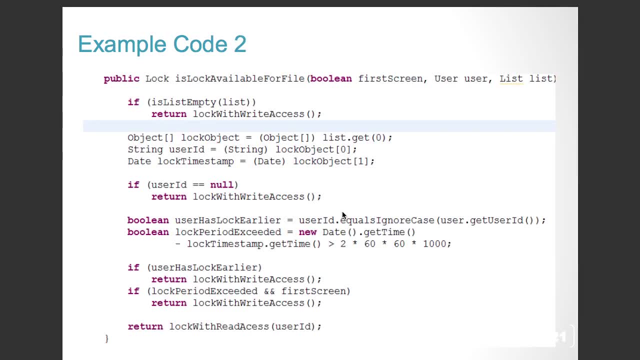 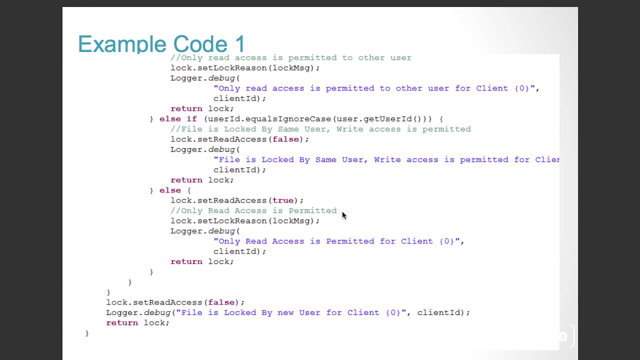 sounds very easy, but the thing is, refactoring is a very, very difficult thing to do. Look at this piece of code. How can you be sure that when you change the code, everything is working as expected? The only way you can refactor with confidence is to build a test. 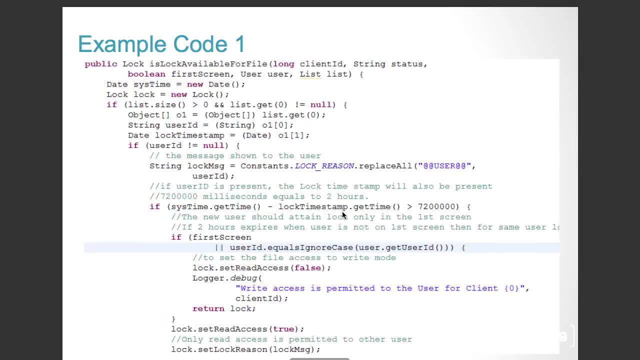 bed. Now let's say I'm doing a very basic refactoring. Let's say I'm renaming a variable or extracting a method. Those are simple refactorings, They can be done safely. But if I'm doing anything complex than that, one of the first things I would do is to check the unit tests and 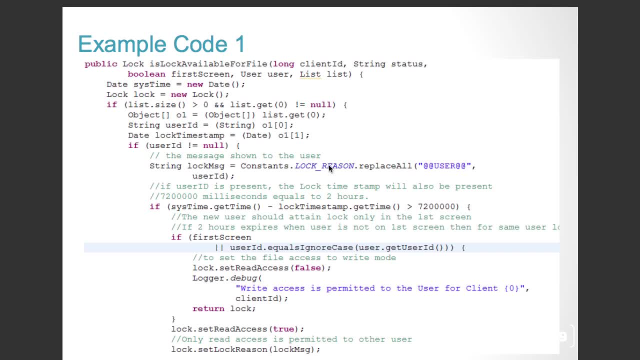 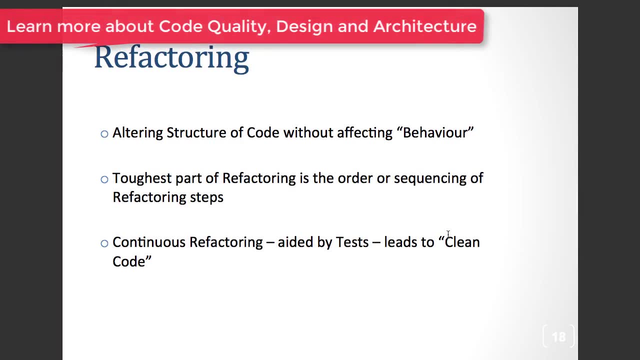 make sure that there are good unit tests available. If there are not good unit tests available, then I would write them. So make sure that you have good unit tests available and only then start refactoring When you have tests. then what you can do is you can improve the code in small steps. 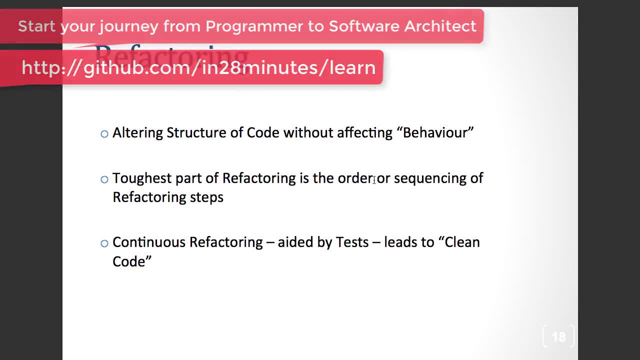 and keep running your tests And after running the test you have feedback whether everything is fine. If everything is fine, go ahead, refactor further. So, as you see in here, continuous refactoring aided by tests leads to clean code. So clean.